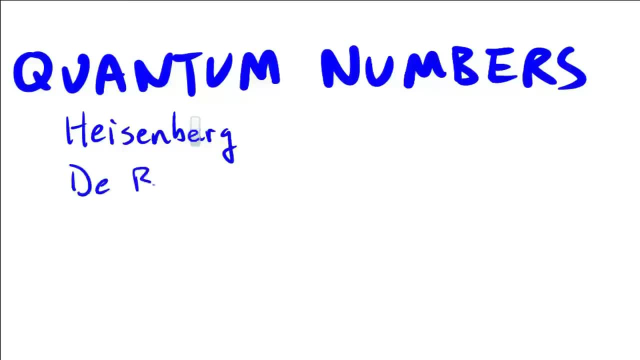 And then you have Louis de Broglie. De Broglie told us that Anything with mass also will have a wave property. But in our everyday experience, things with mass like people or soccer balls don't seem to have any wave properties whatsoever. 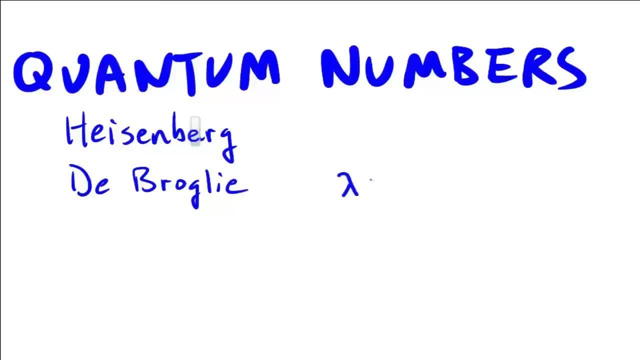 And that is because the wave property, which we will symbolize with the wavelength, is inversely proportional to the mass. And so if you have a very, very, very tiny mass, like an electron, Then the wavelength or the wave property of that particle becomes quite significant. 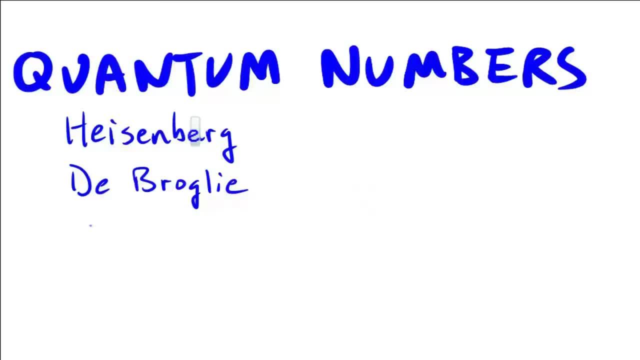 And so then, with that in mind, we have Schrödinger. Erwin. Schrödinger was umlauts. He came along and defined what the electron is doing inside the atom, based on it being a wave and not a particle. And he defined what the electron is doing inside the atom, based on it being a wave and not a particle. And he defined what the electron is doing inside the atom, based on it being a wave and not a particle. And he defined what the electron is doing inside the atom, based on it being a wave and not a particle. 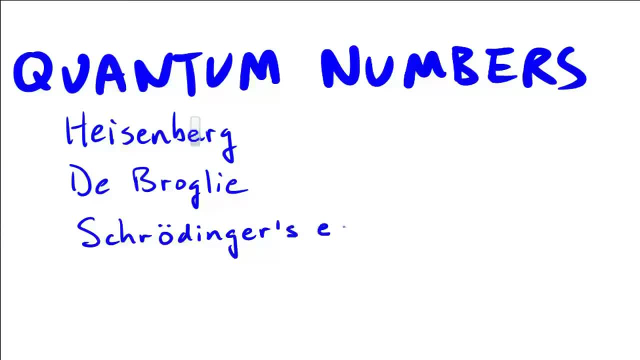 doing mathematically, and so we call that Schrodinger's equation. Now, the equation is very complicated math, but we can derive from the equation three quantum numbers symbolized: n, l and m sub l, as well as a fourth that came a little later, m sub s, and we will take a look at these in. 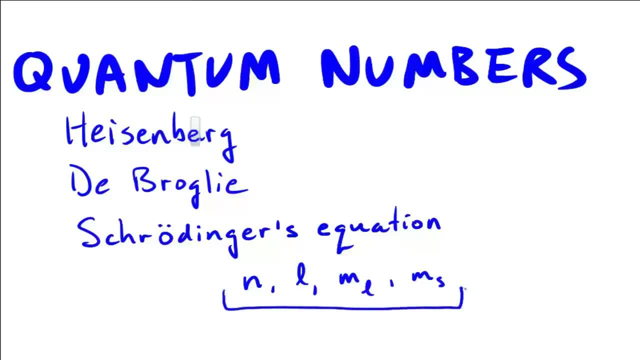 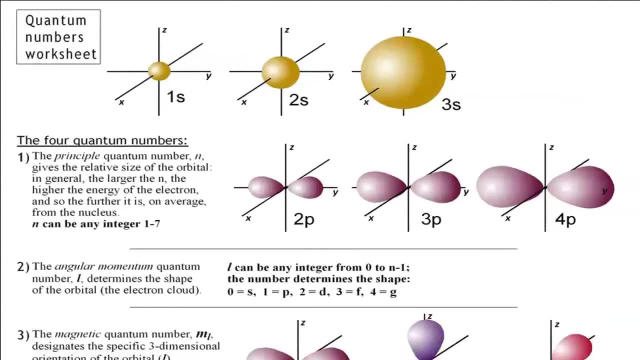 the rest of this presentation. What do each of these symbolize and how are they related to what the electron is doing, what the orbitals are and how the orbitals are oriented? Okay, so let's take a look at s-orbitals and p-orbitals. First up, the s-orbitals. As we know, orbitals. 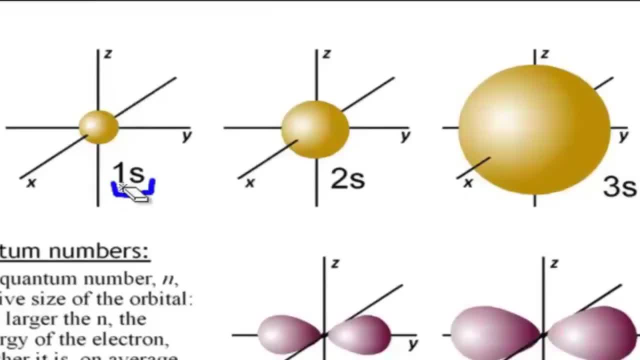 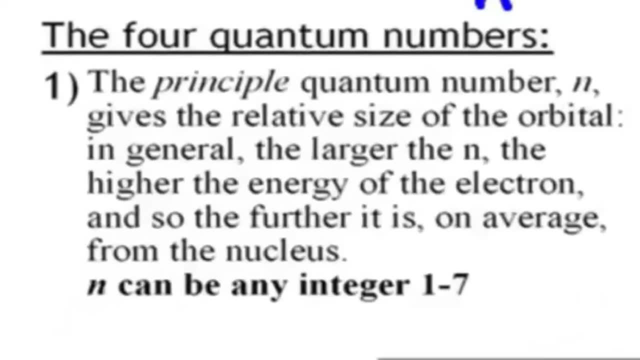 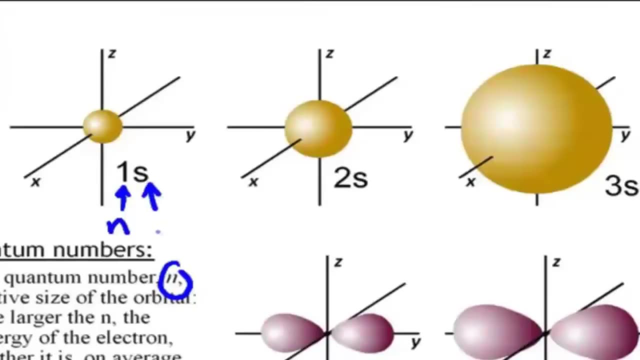 are always represented by a number and a letter. Well, the number is the principal quantum number, and that is our first quantum number symbolized as n. The letter is our second quantum number, symbolized as l, and that tells us the shape of the orbital. 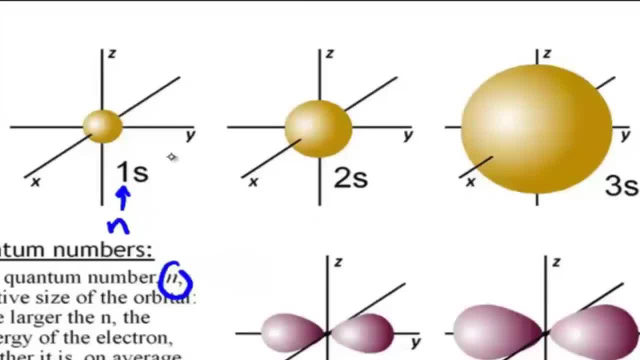 But we are going to not talk about the shape at this moment. we will a little bit later. Let's first take a look at what the principal quantum number tells us. Here we have the principal quantum number going from one to two to three, and what happens to the orbital. 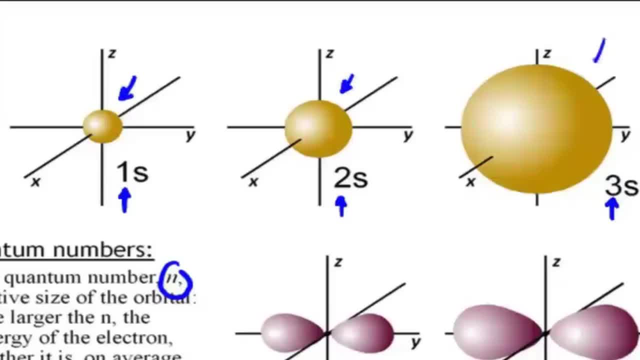 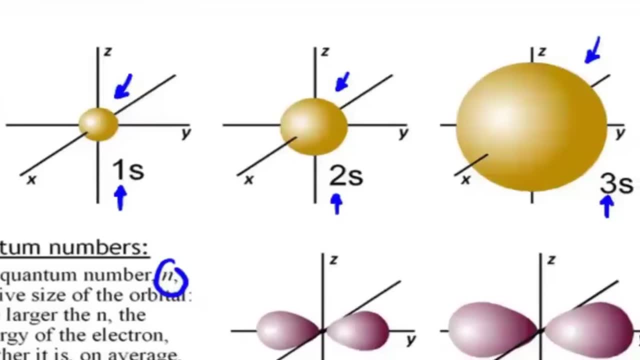 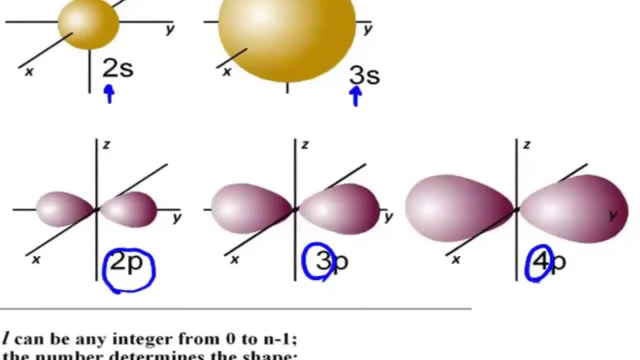 as we go from n equals one to n equals two to n equals three. It gets bigger. As n gets bigger, the orbital gets bigger. If you look at the p-orbitals: two, p, three, p, four, p on n equals two. we have this sized orbital: n equals three, a bigger orbital, and n equals. 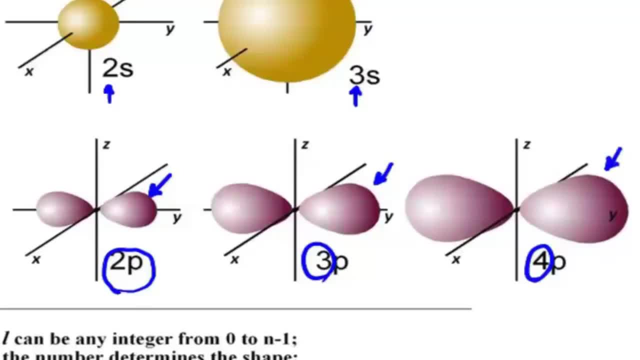 four, an even larger orbital. So there is a direct relationship to how far away the electron is from the nucleus and the principal quantum number. That is because the energy of the electron increases as the principal quantum number increases and because the electron has more energy on average, it is going to be further from the nucleus. 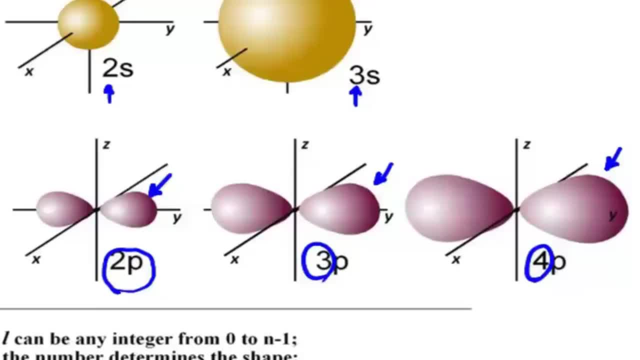 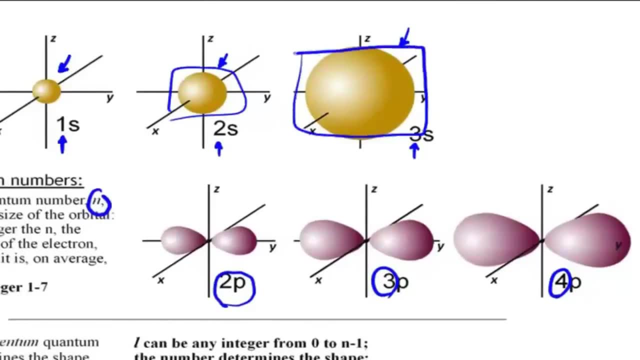 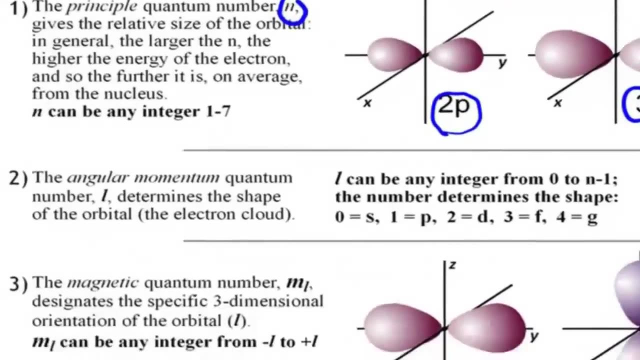 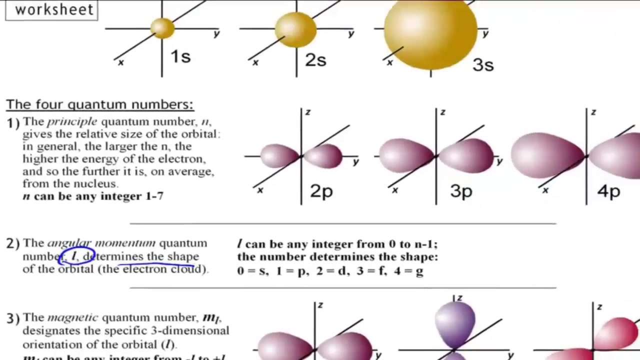 And therefore occupy a space that is larger, and that larger space is shown here as the surface of the orbitals getting larger. Now let's take a look at l, the angular momentum quantum number. This determines the shape of the orbital and, as you can see, the s shape. 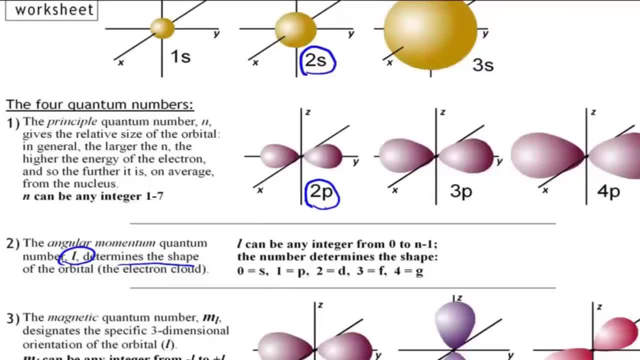 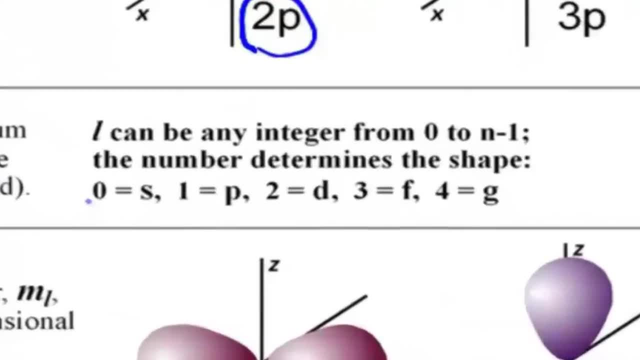 is quite different than the p shape, But we are talking about quantum numbers, not letters. So in fact each letter has a corresponding number. Zero represents the s orbital. when l equals one, that is the p orbital. l equals two is the d shape, three is f, and when l equals four, we have g orbitals. Note that. 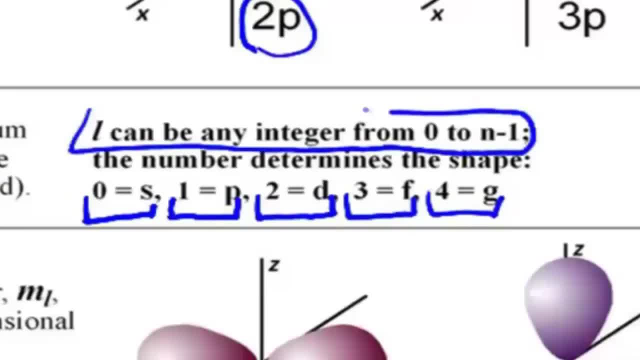 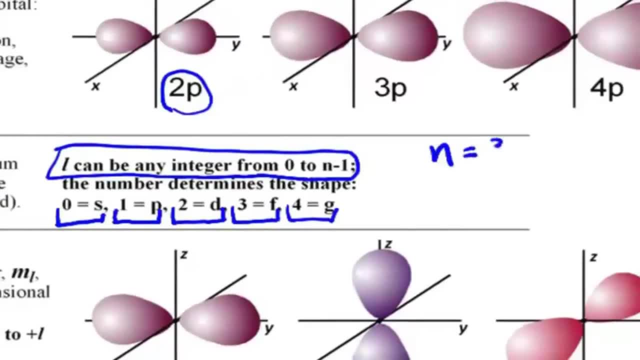 l can be any integer from zero to n minus one. So, for example, if we have a principal quantum number of three, then L can have any shape, from zero, which is s, or one which is p, or two, which is d. 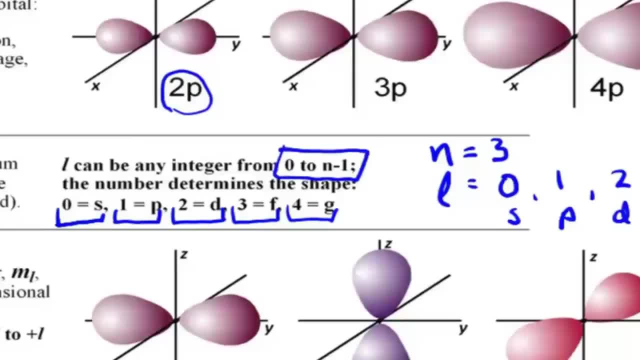 So that zero, one and two are zero to n minus one. What about if n equals two? L can be any orbital from zero or one, in other words s or p. And if n equals one, L can only be zero or s. 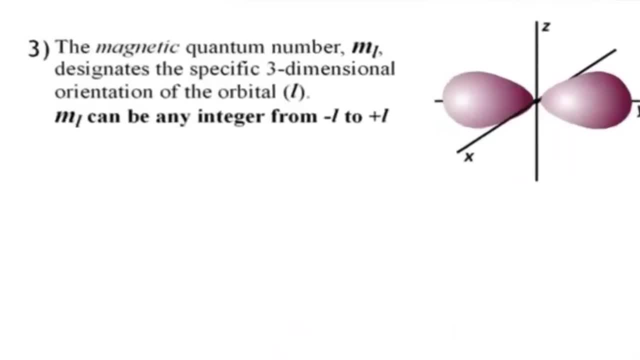 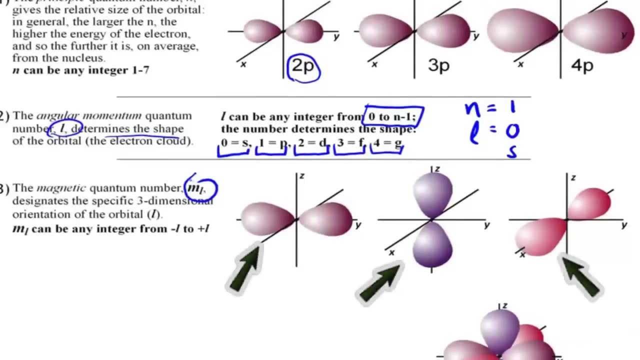 And the third quantum number, the magnetic quantum number m sub L. Here we can see that the three p orbitals exist in different orientations in three-dimensional space, and that is what the magnetic quantum number m sub L is telling us. M sub L equals one. 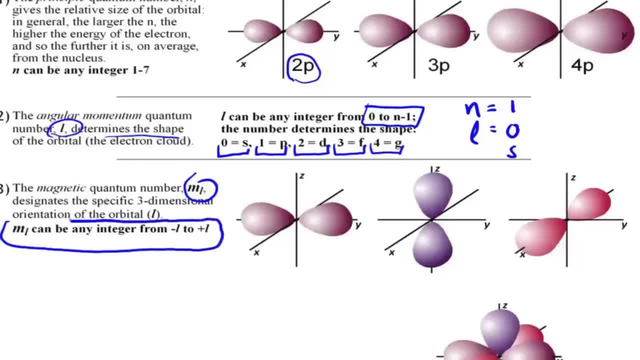 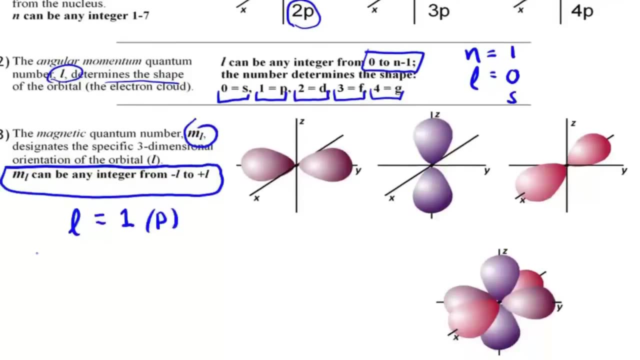 M sub L can be any integer, from negative L to positive L, and each integer represents a different orientation in space. For example, if L equals one, in other words p, then m sub L can be any number, from negative L to positive L, any integer. 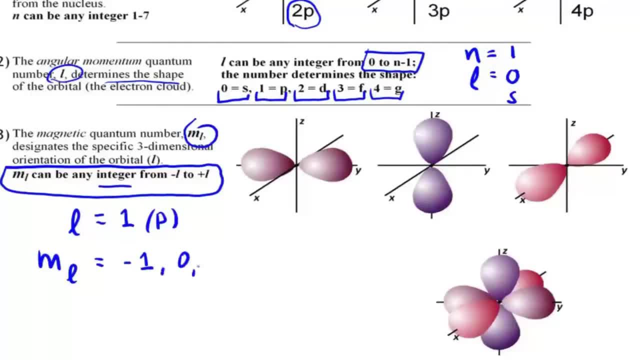 And so, therefore, we have negative one, zero and positive one, And so, therefore, we have negative one, zero and positive one as possible. m sub L numbers, That's a total of three numbers, and that's exactly how many orbitals we find in the p. 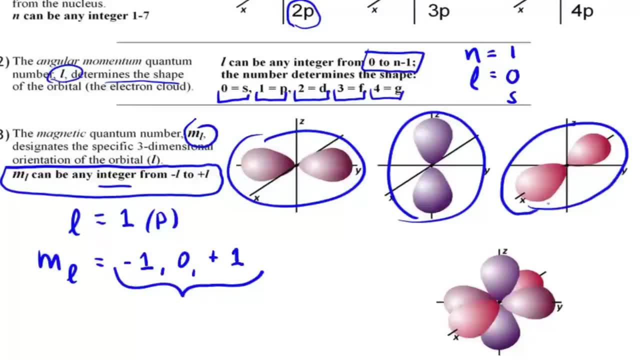 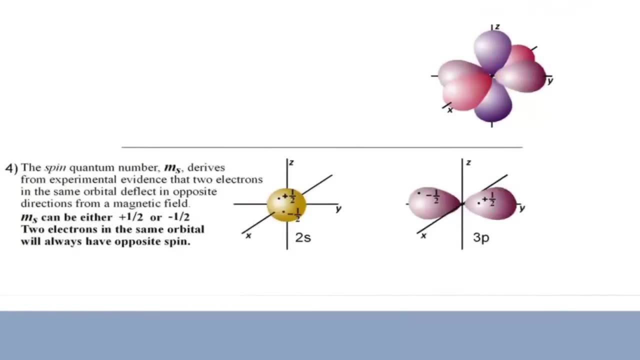 orbital at any one energy level And these three orbitals are oriented perpendicular to each other on the x, y, z axes, and we can see that when you look at the three orbitals simultaneously. And finally, we have the spin quantum number m sub s. 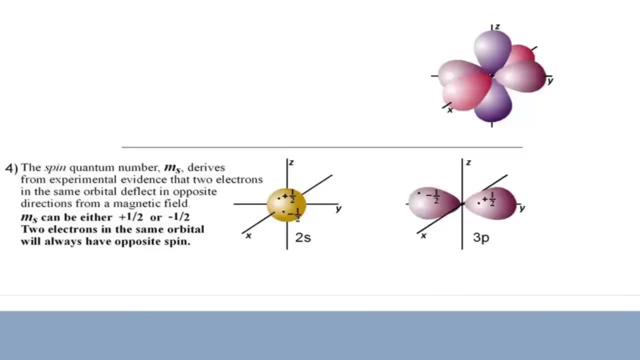 And this derives from the fact that, experimentally, electrons in the same orbital are found to deflect in opposite directions when going through the same magnetic field, And those two electrons are designated as either positive one-half or negative one-half. They are said to have opposite spin. 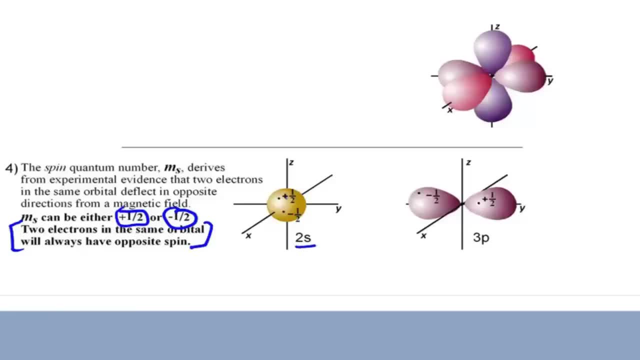 So, for example, in the 2s orbital, let's say you have two electrons, One will have a spin of positive one-half, The other one will have a spin of negative one-half. Another example: 3p. If there's two electrons in one of those 3p orbitals, they will have opposite spins- positive. 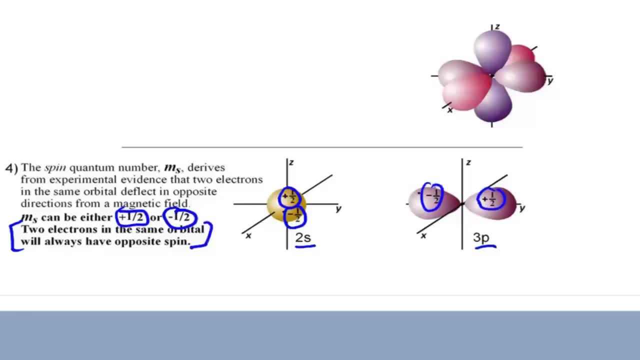 and negative one-half, And the spin quantum number allows us to say that no two electrons in any one atom can have the same set of quantum numbers. For example, let's look at the quantum numbers That represents The two electrons in 3p. 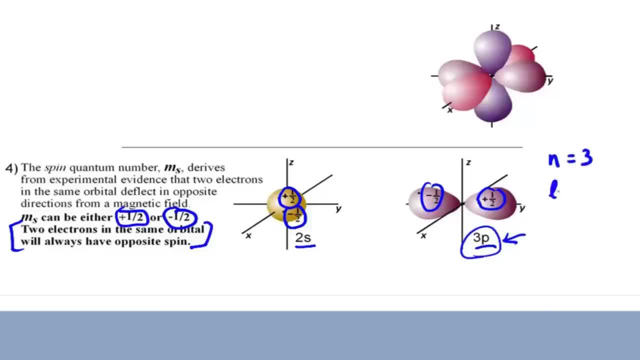 N equals 3, when in 3p L equals 1.. That's p right. M sub l can be anywhere from negative, one-zero or positive one. We'll just pick one and say it can be zero. So what is going to distinguish these two electrons? finally, is the m sub s? 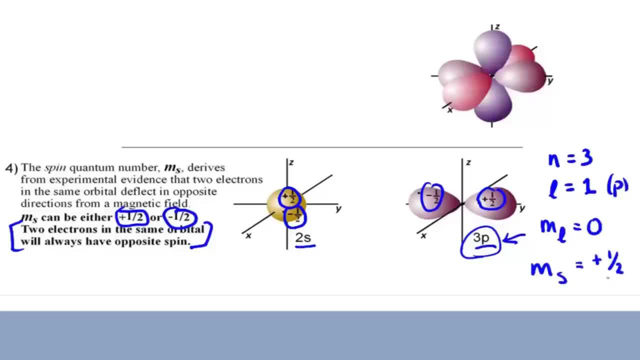 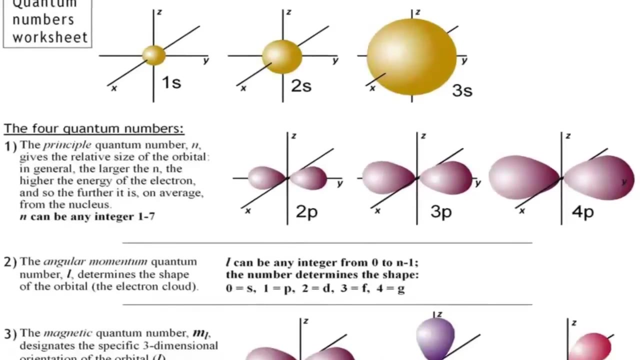 One of them will be positive one-half and the other one will be negative half one-half, And so you'd never have two electrons with the same four quantum numbers in an atom. One very, very important thing: we need to lay a misconception to rest, and that is that 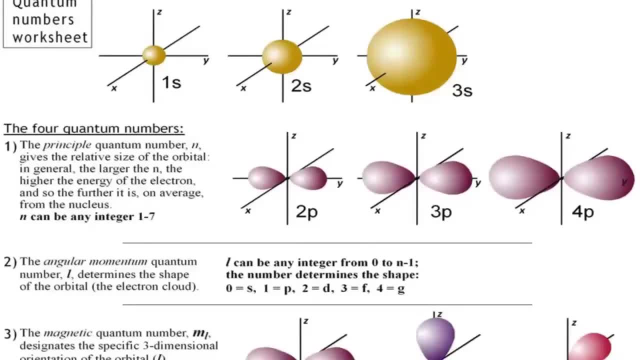 the principal quantum number, also called the principal energy number, represents the actual energy of the electron. That is only true in hydrogen and every other element. that is not true the energy of the electron. This is represented by both the principal quantum number as well as the angular momentum. 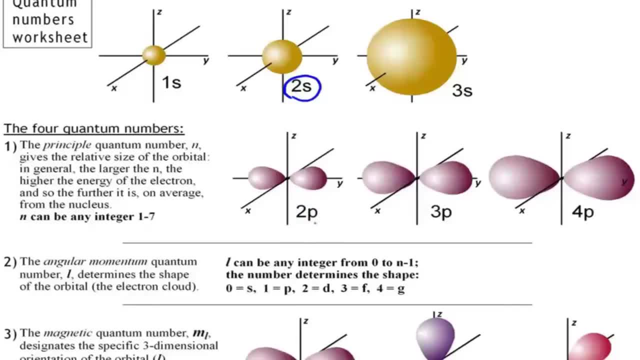 quantum number l. So the l value- in this case one, and the n value- in this case two- together represents the energy of the electron. So a 2p electron will have a different energy than a 2s electron. 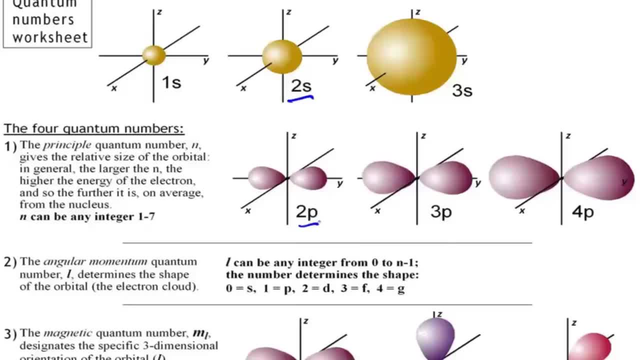 So that's it, Thank you. Hydrogen is different because it only has one electron. There are no repulsions, there's no penetration of electrons to the nucleus in a single electron atom, And so it is only the principal quantum number that actually designates the electron's energy. 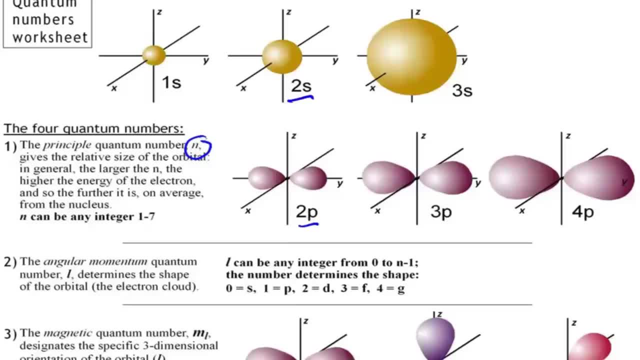 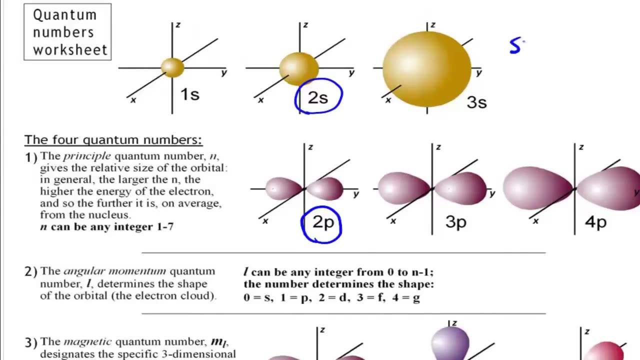 in the hydrogen atom. Once you have more than one electron, you start getting these repulsions and penetrations and that separates the energies of the electrons in the different orbitals. And an important term that we should take a look at is the word sublevel. 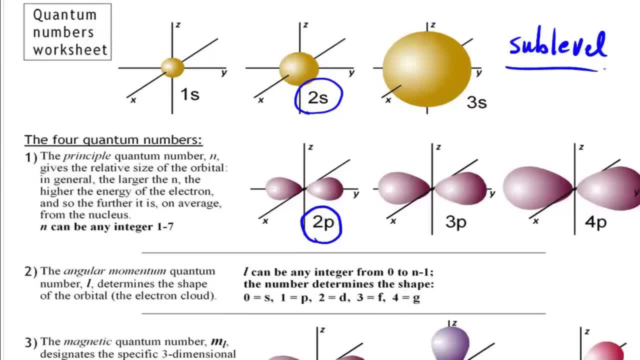 And sublevel is commonly used to refer to the specific orbital that an electron is existing in. For example, you can have an electron in the sublevel 2s or 3s or 3p, And so the sublevel refers to both the principal quantum number as well as the angular momentum. 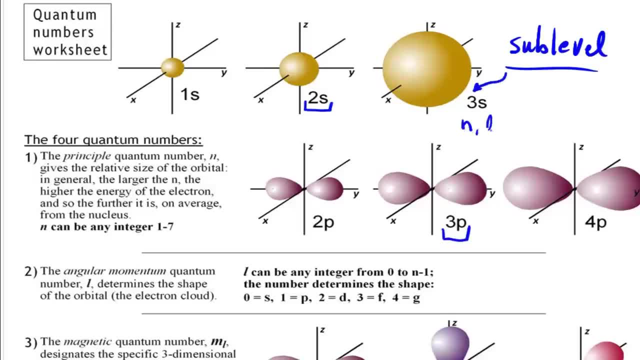 And this is what we call a sublevel, And when you think about it, you think about the principle quantum number. the principle quantum number as well as the angular momentum, the L-value together, And so therefore, the sublevel represents the energy of the electron in any element. 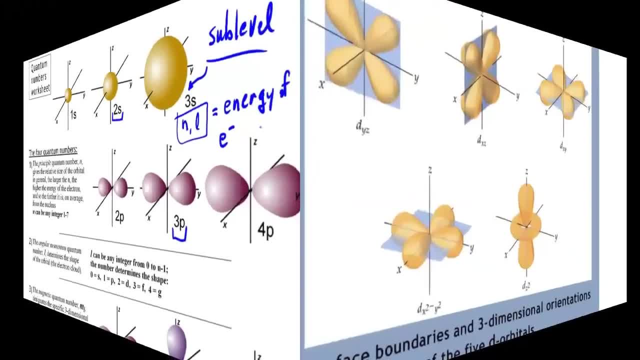 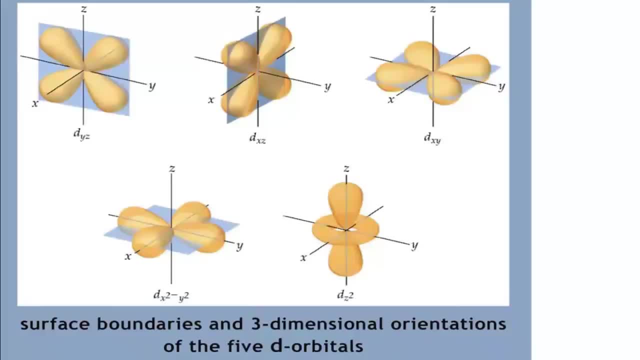 other than hydrogen. Let's take a look at the surface boundaries and three-dimensional orientations of the five d-orbitals. So here again, presented on the x, y, z axes, we can see that every one of these orbitals has a different orientation in three-dimensional space. 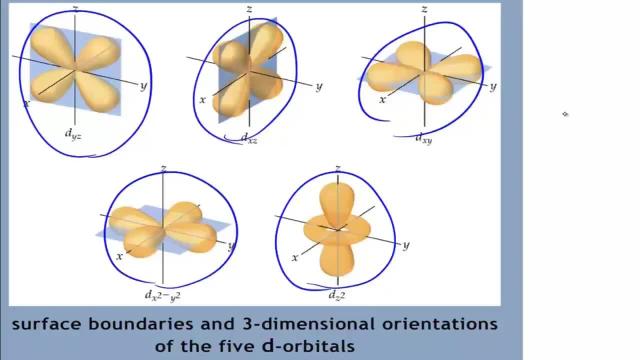 So notice that there are five orbitals at the d-level and we can use quantum numbers to understand why that would be the case. We know that at the d-orbital the quantum number is two And the orientations m sub l are going to be negative l to positive l. 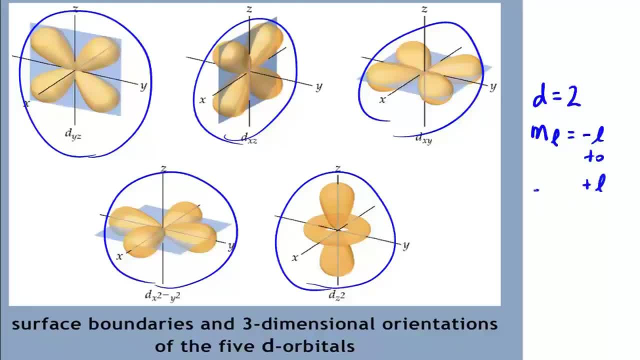 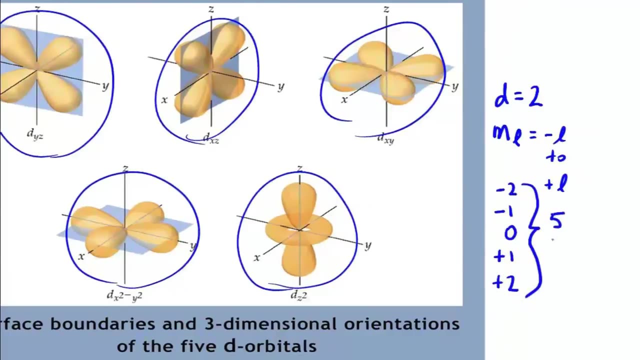 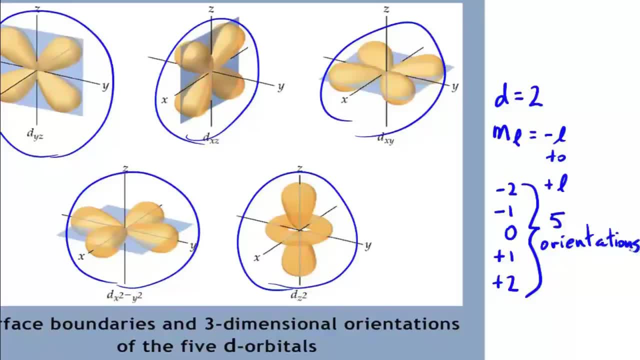 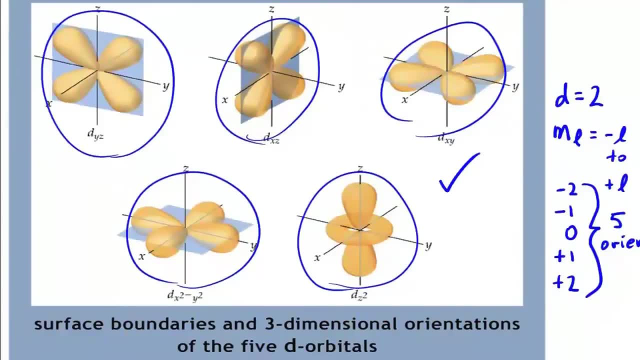 There's five possibilities of d-orbitals in three-dimensional space, for orientations of d-orbitals in three-dimensional space, And that's exactly what we see: Five orbitals at any one energy level. Let's take a look at the surface boundaries and p-dimensional orientation of the seven. 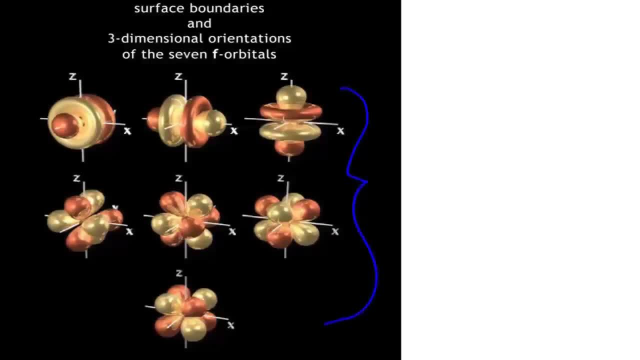 f orbitals. Here we're given an illustration of the seven f orbitals and we know that, for the l value, f is equal to 3.. and that we know, therefore, with M sub L being equal to anywhere from negative L to positive L,